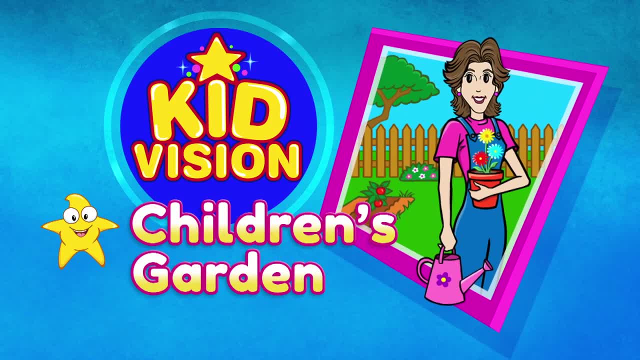 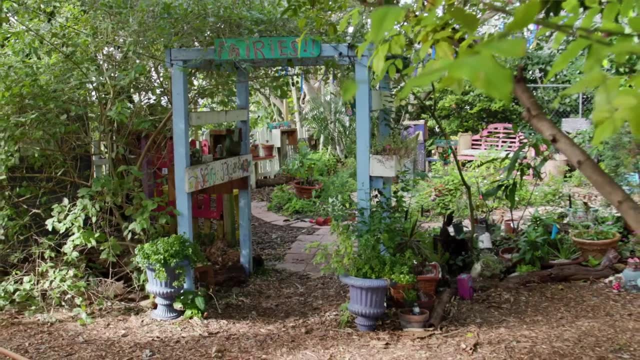 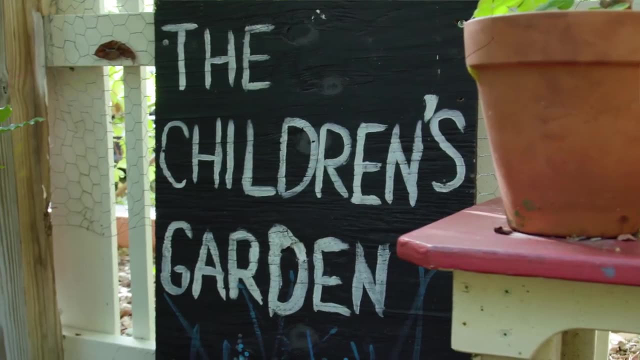 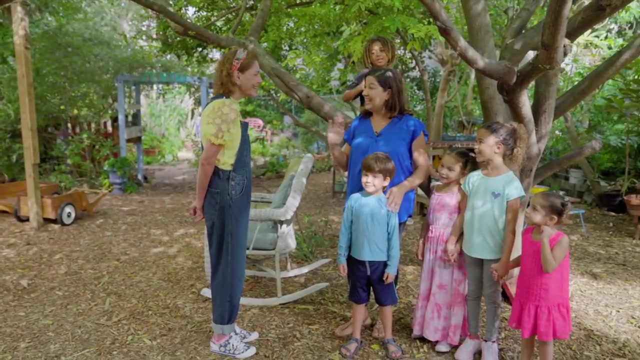 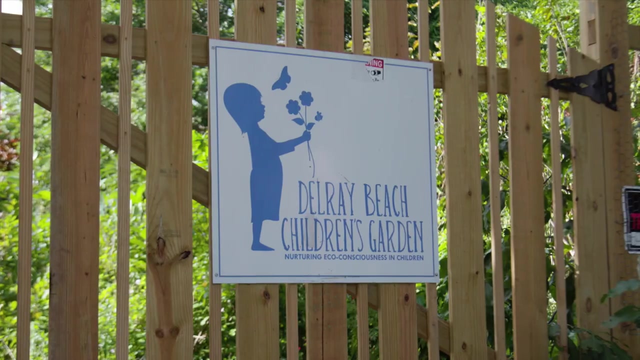 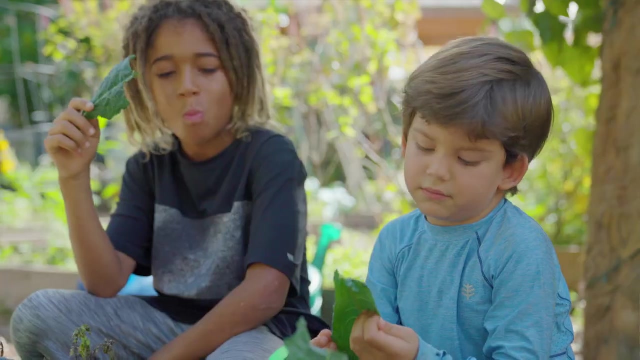 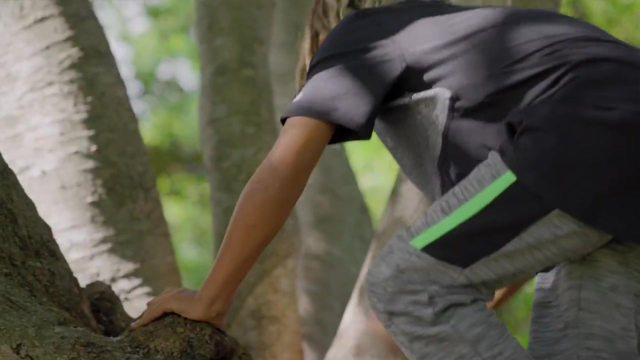 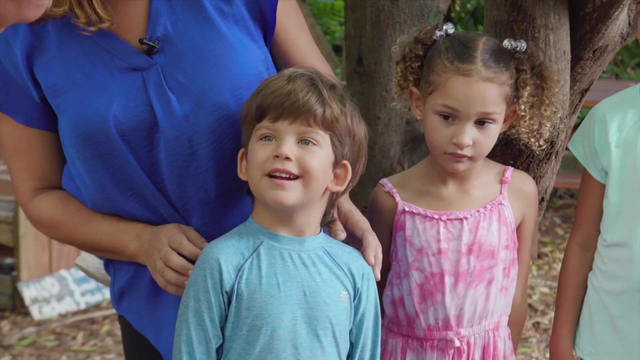 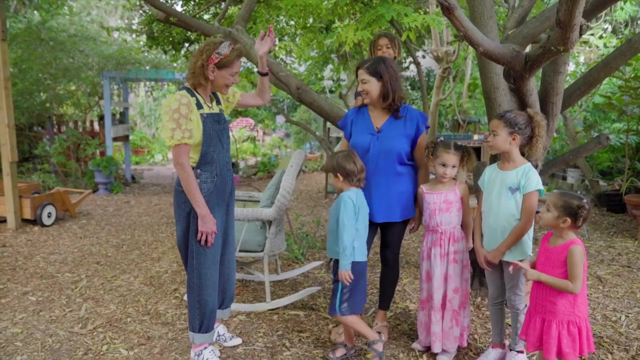 Hello, Hi, Miss Penny. Hi, Welcome to the children's garden. It looks amazing. Tell me about it. Well, this is a garden built for children, by children, And it's a really beautiful place for children to play outside, learn about our ecosystem and grow food. Oh, it sounds amazing. I can't wait to play with you. What's your favorite part? The strangler fig tree over there. Do you climb it? Yes, Sounds fun. What's your favorite part? The berries and the tree right here that I'm standing under. Oh, this tree we're standing under and it has berries. Yeah, I'm just gonna look for berries. 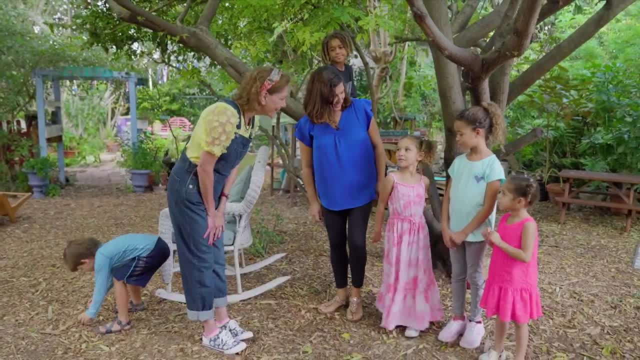 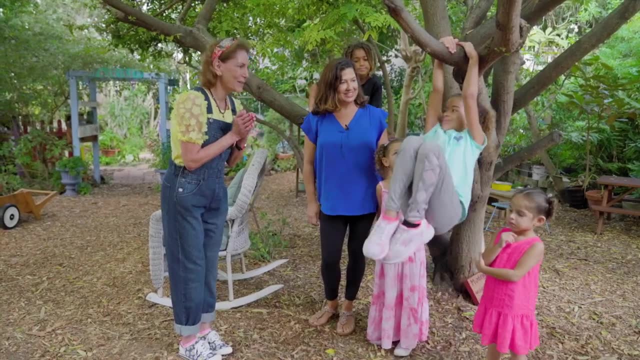 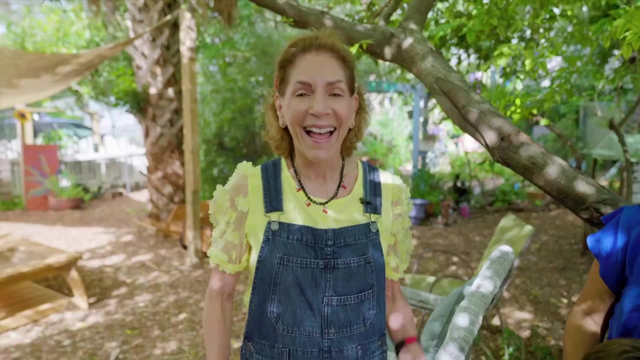 It's berries, Okay. And what's your favorite part? Water play. Oh, I love water play. We get to do that today. And your favorite part: Trees, Trees. Everybody loves trees. And what's your favorite part? Mug kitchen. Oh, the mug kitchen. I can't wait to explore this whole garden. Follow us, Miss Penny. Oh, I will, Let's go. 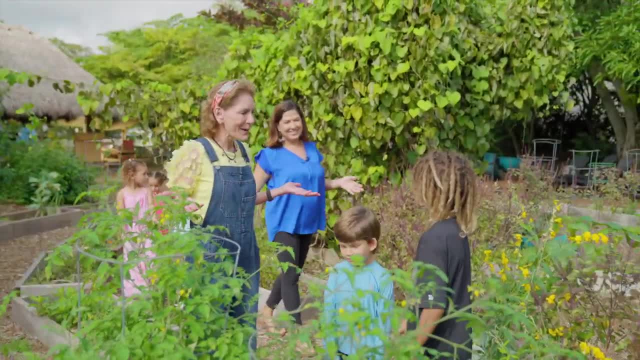 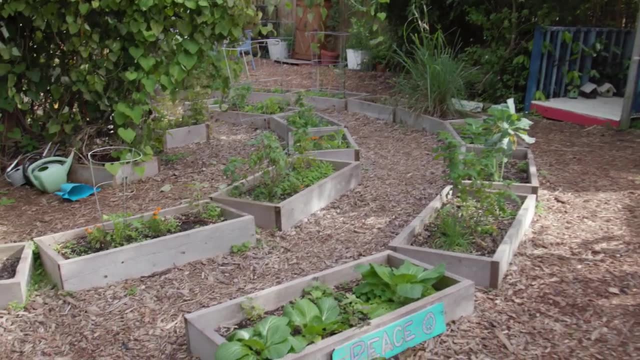 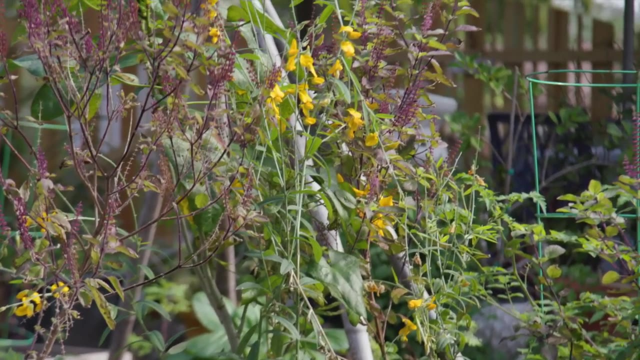 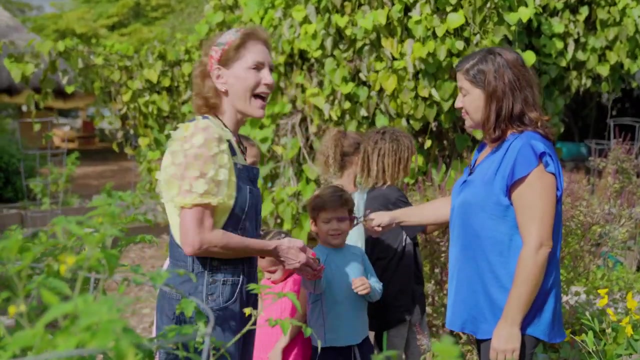 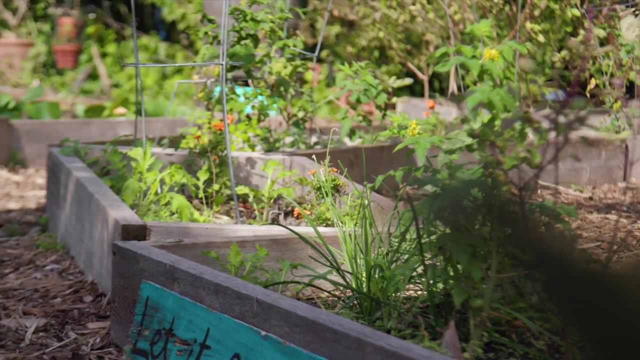 Wow, Is this cool. What do you call this part of the garden? Our veggie maize, Your veggie maize. So you grow vegetables here And growth right here tomatoes, Tomatoes and what other kinds of vegetables? Lavender, basil? Oh Smell, Wow, That smells amazing. And you grow it. Do you help grow the garden? Yeah, What do you do? 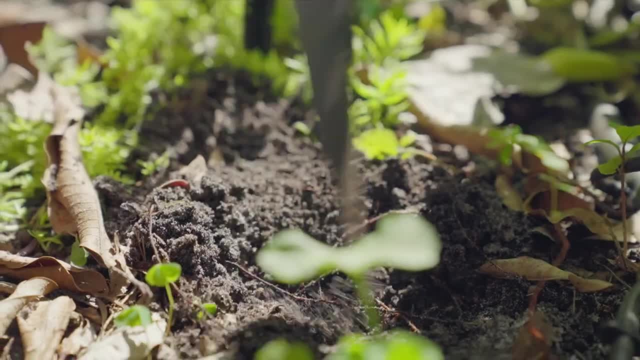 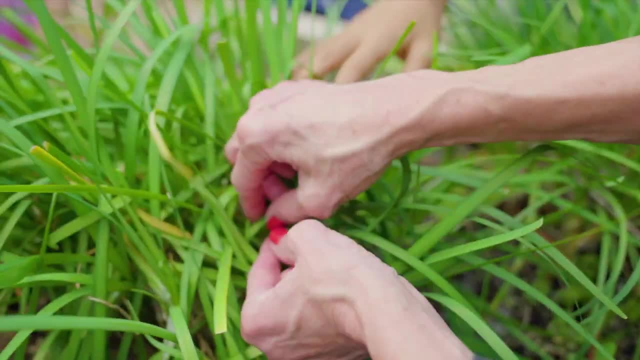 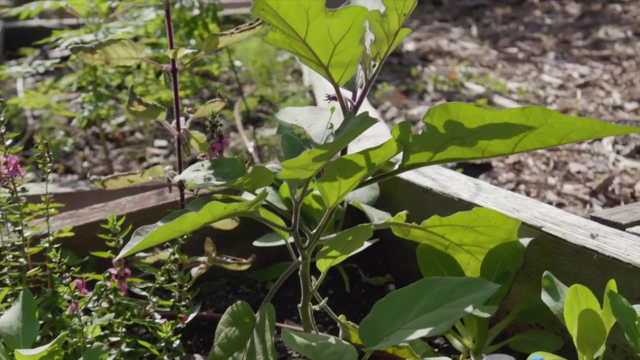 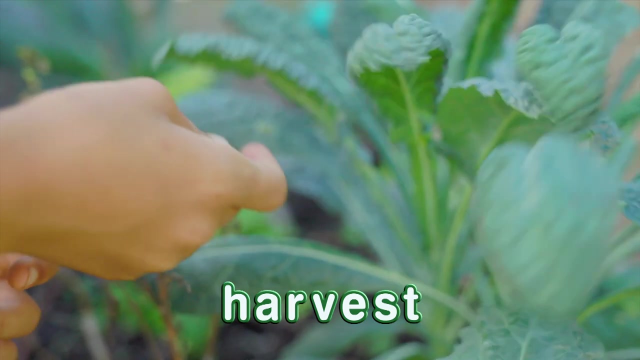 here, I just sprinkle seeds. You sprinkle seeds and then you water them and then you take care of them and watch them grow. Yes, The children plant all the vegetables and herbs here and then we harvest them to use them in our plant-based meals that we prepare here. Harvest is a good word. What does that mean? Well, it means that when the fruit or vegetable or herb is ready, you pluck it from the plant and you use it to nurture your body. That's terrific. And how do you know when a plant 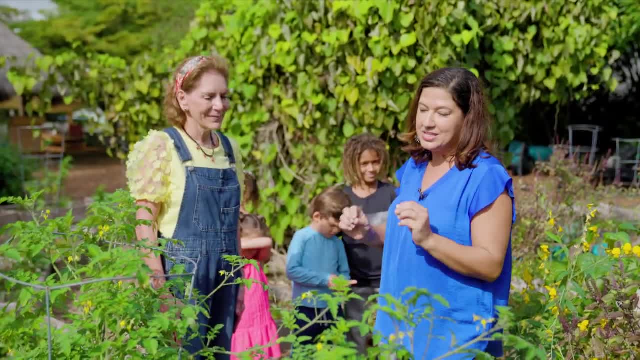 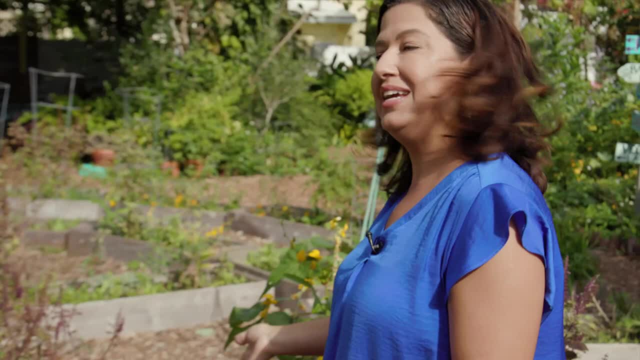 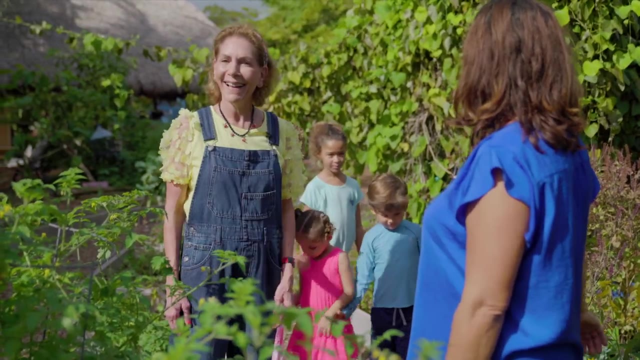 is ready Well, for a tomato, for instance, it's when it's nice and bright and red and plump. Sometimes they're yellow. And for other things, like greens, it's when they're a nice medium or large size. That's wonderful. And then you do cooking. How great is that? It's amazing, I think. 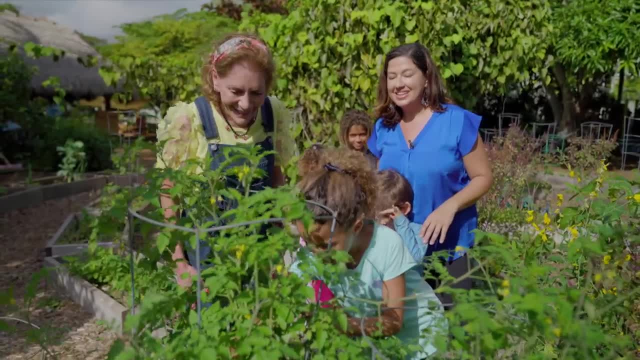 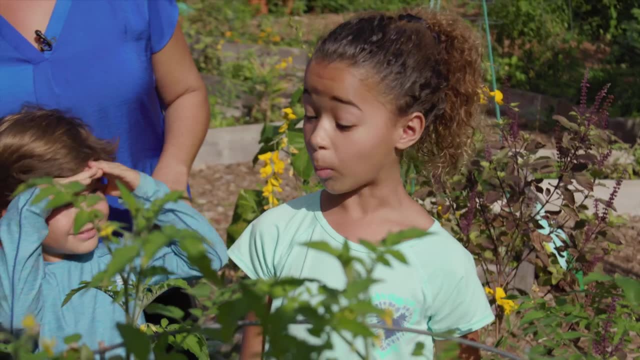 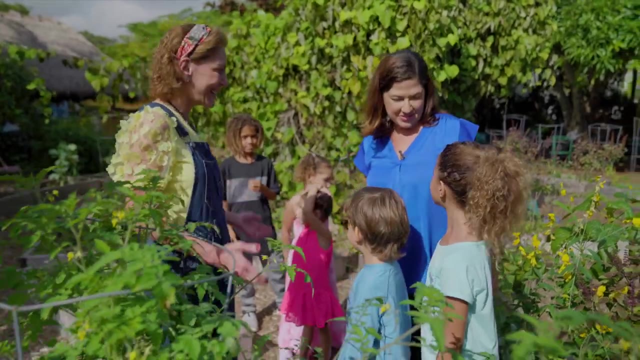 there's a juicy tomato right there. Oh, my goodness, Are you going to eat it? It's good, Very, Yay, Good job. This is an amazing garden. Sweet tomatoes- Oh, it's a sweet tomato. That's fine one for you too. 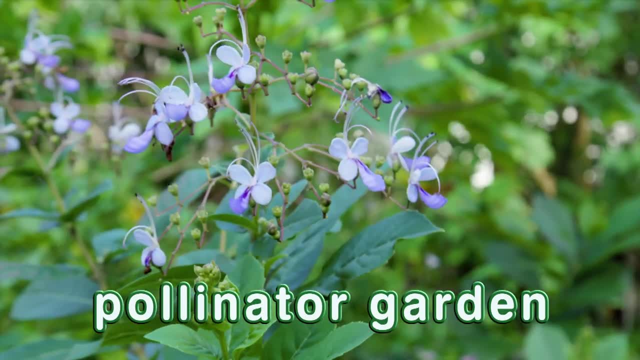 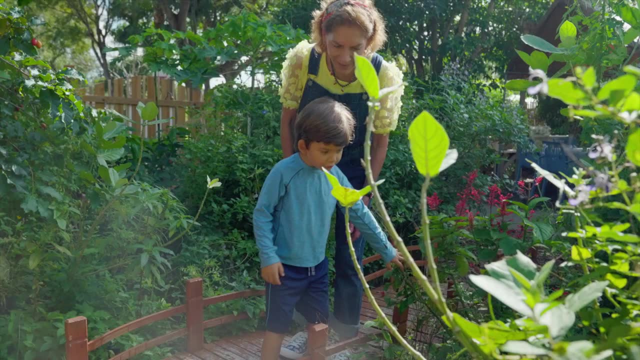 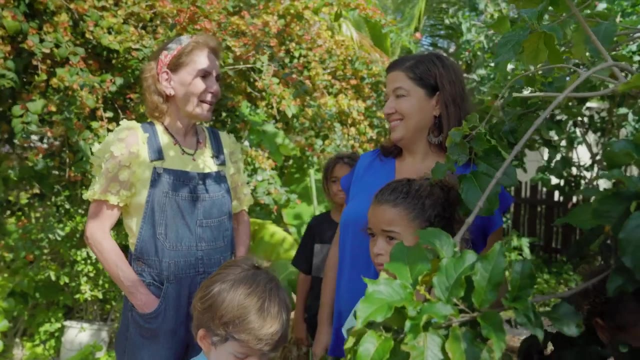 We call it a pollinator garden Because all of these pollinator plants attract butterflies, bees, dragonflies, hummingbirds. Pollinators are really important. They help drink nectar from each plant and carry it to one another so that plants can grow and fruit- Very important Without them. 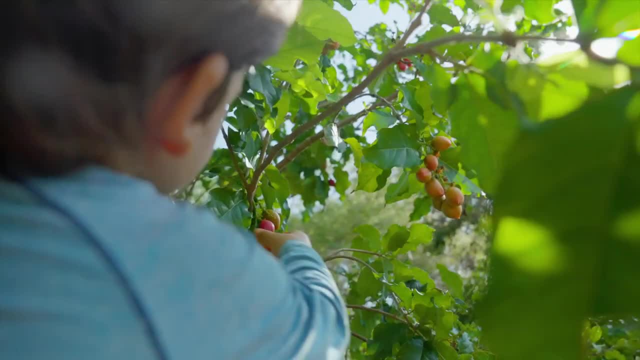 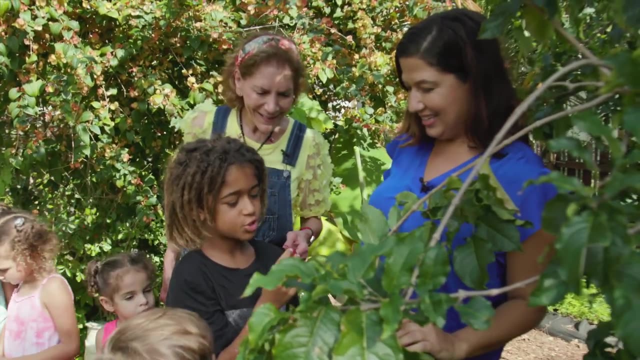 we wouldn't have plants and fruit. Exactly, And I see this tree has berries on it. It does. This is our peanut butter fruit tree. Peanut butter fruit. Want to give it a try? Do you want to taste this? Do you want to feel it? 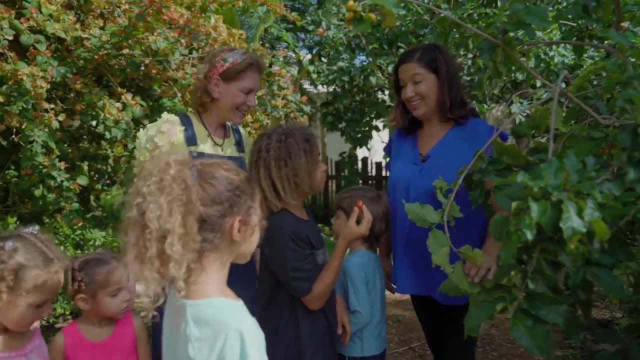 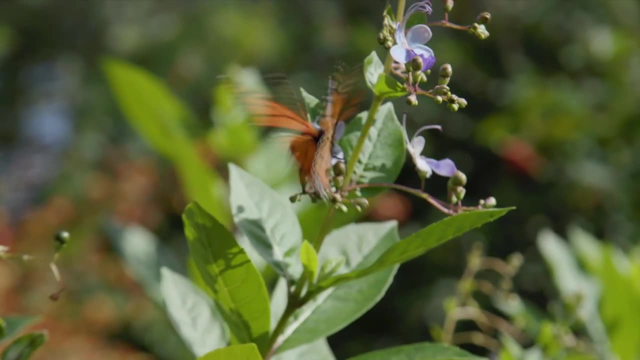 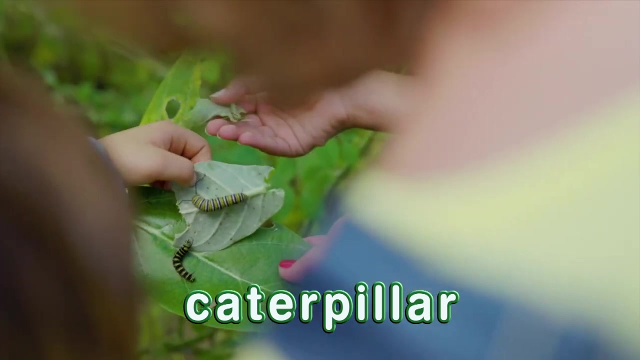 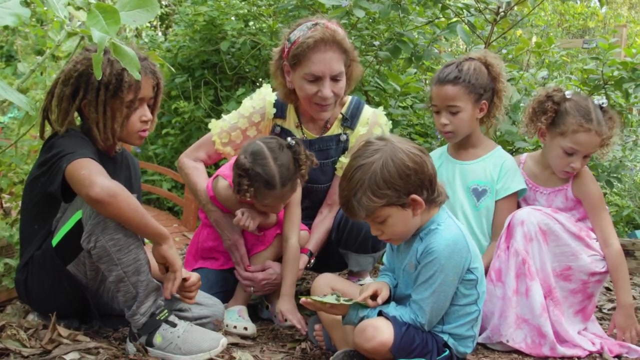 It's strange. It's like peanut butter. You want to feel it Surprising? What is this animal called? It's a caterpillar, Caterpillar, And we have all sizes and shapes of these caterpillars- Yeah, Black, white. 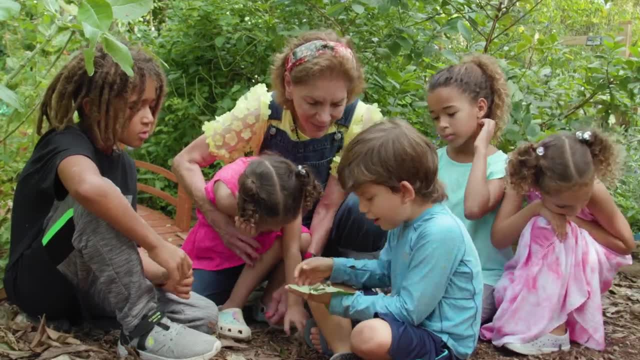 There are those colors, and then can you count. Count one One. Yeah, Let's count One One. No, No, Nope, Don't eat it. Don't have to eat it, Not that one. It's good, energizing, Ouch, It's so good. 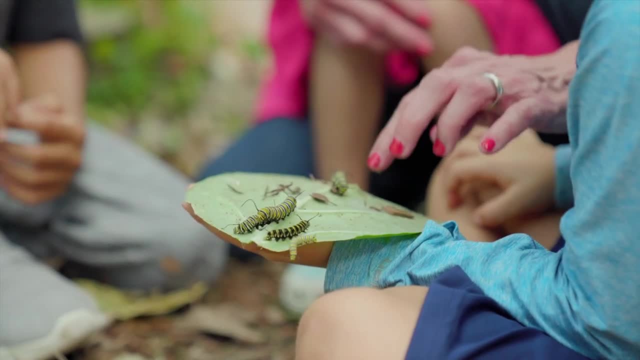 Good job norms, Gotta clean. Yeah, Do it. Well. I'm so thrilled It loves it. I love the permission to have her. Let's count One, two, three, four, five caterpillars on one leaf. That's pretty cool. 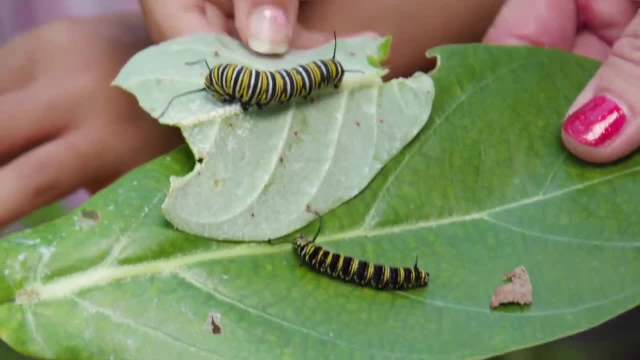 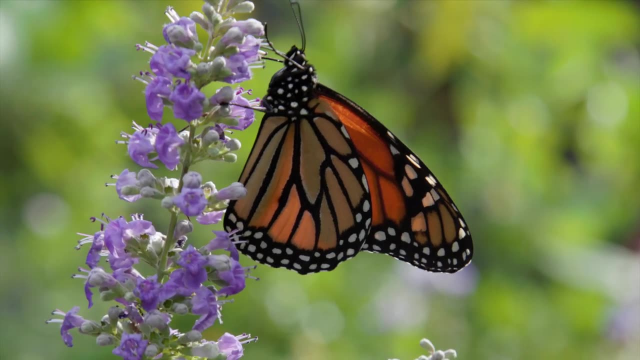 They live on milkweed. They live on milkweed And we're holding milkweed. What are they going to turn into after their caterpillars? A monarch butterfly, A monarch butterfly. I think it's time for some nature play. Let's play with nature. 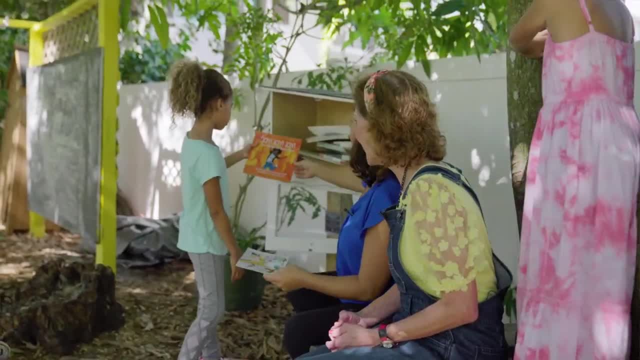 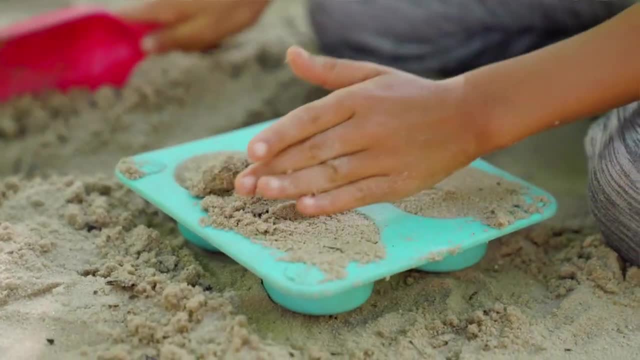 One of the really awesome parts of the children's garden is that the children make their own decisions. They play how they want to play with what they want to play with. So they really roam free, even though it's a safe space, and feel like they're out in the wild. 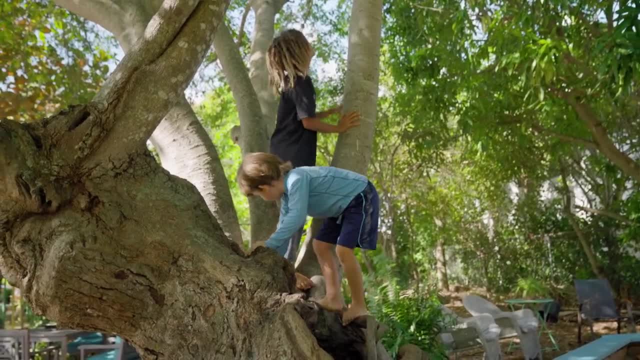 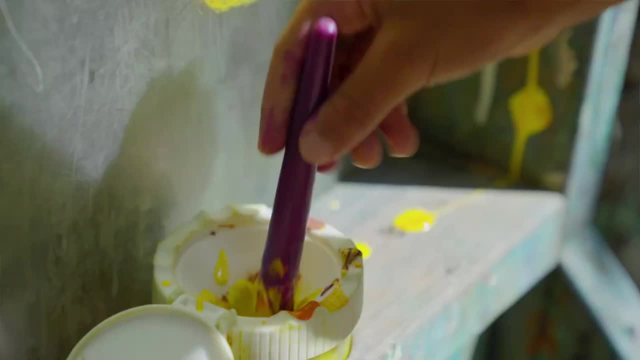 What I love about this place is that- trees to climb and fairy gardens, And it's just you use your imagination. it could be anything you want it to be. Definitely There's a lot of space for your creativity, learning, tasting. 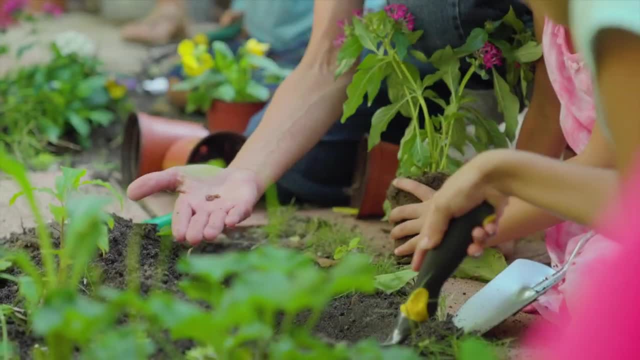 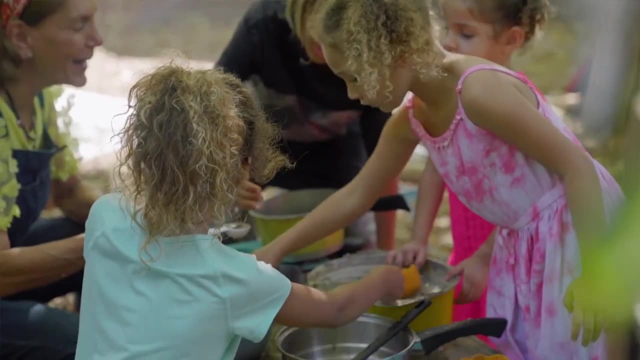 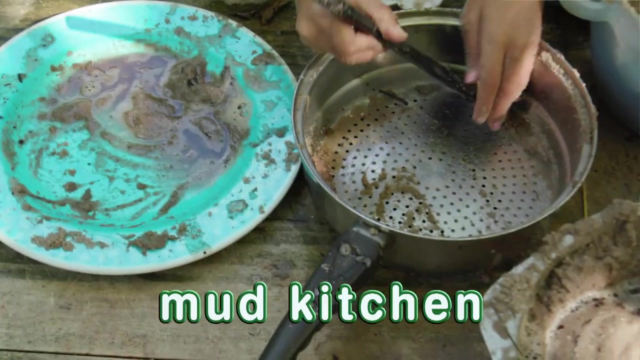 and learning how to be stewards of the earth, how to take good care of our earth. Yes, You really see children from all over our community, different ages, different backgrounds, and everybody comes here to have fun in nature. A mud kitchen is a kitchen where you get to use your imagination to make food out of mud. 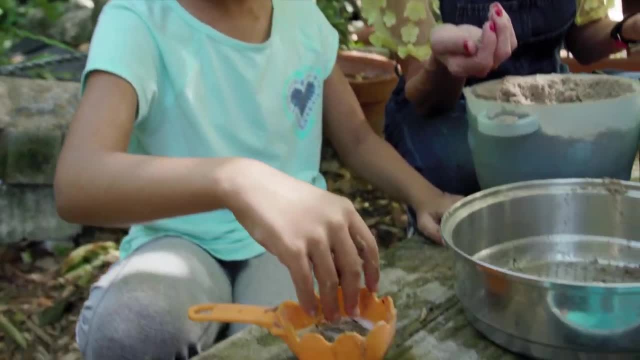 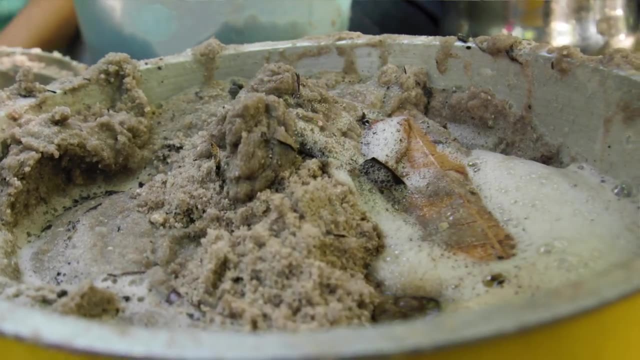 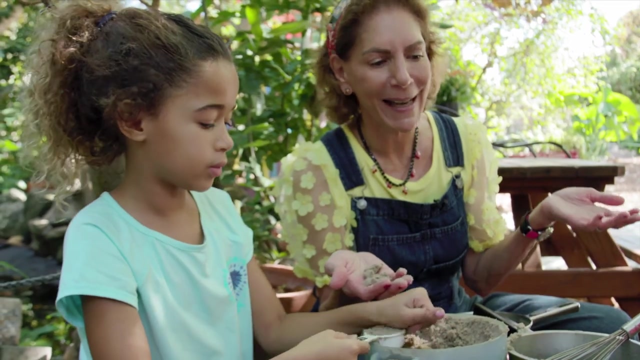 So you use your imagination and you get to get nice and messy and playful, right Yeah. And what ingredients are you putting in? Mud, Mud And a little bit of soap and a little bit of water and it turns into sugar and spice and everything nice. 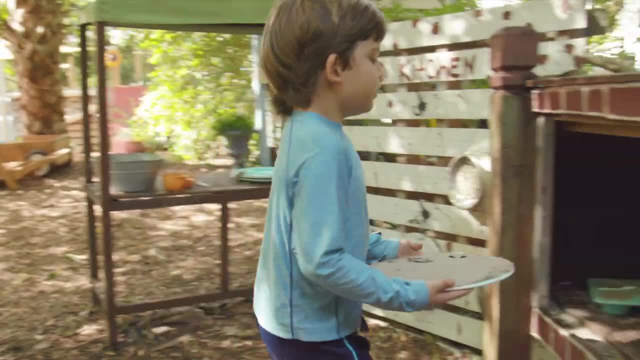 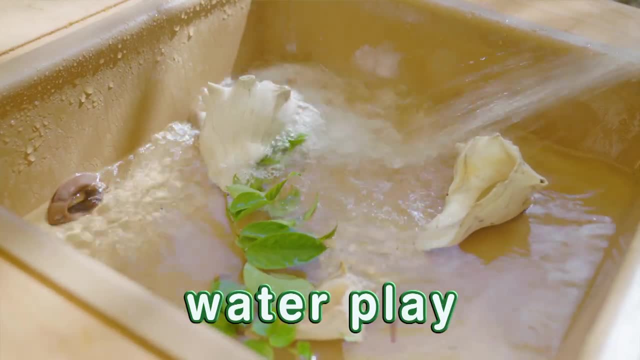 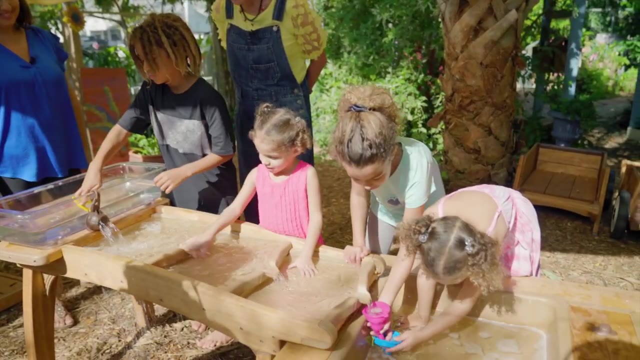 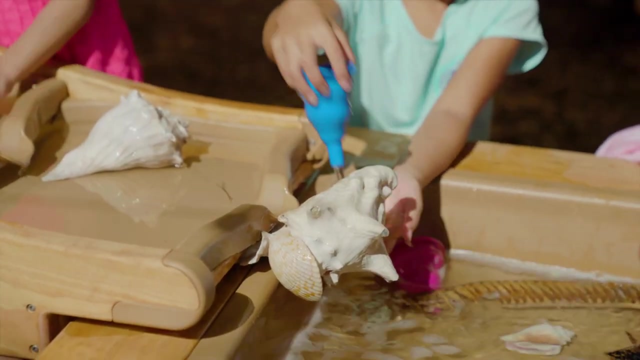 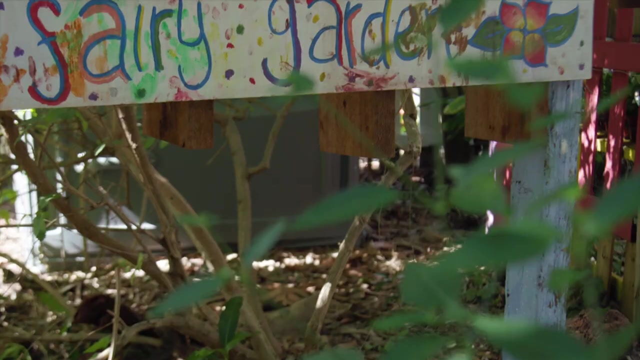 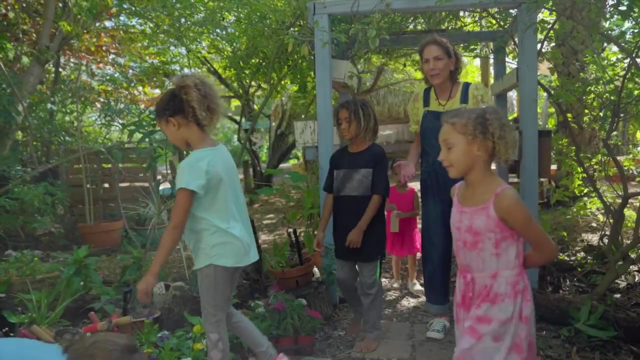 Yep, The waterfall is a peaceful waterfall. Oh my goodness, that's beautiful. I feel the peacefulness from it. It's also a great place to keep cool. I mean all the fairy garden. It's so beautiful in here. Look at all the treasures. 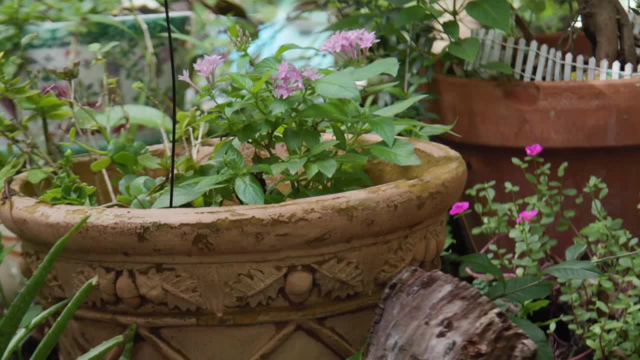 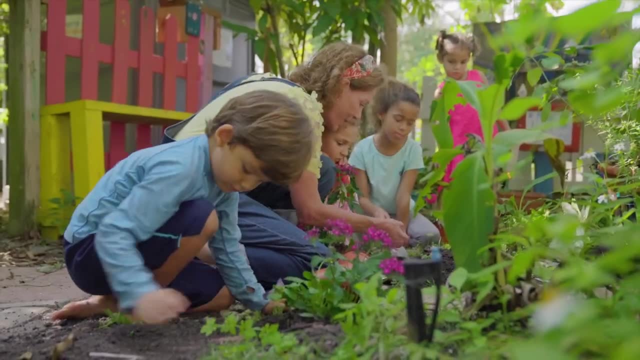 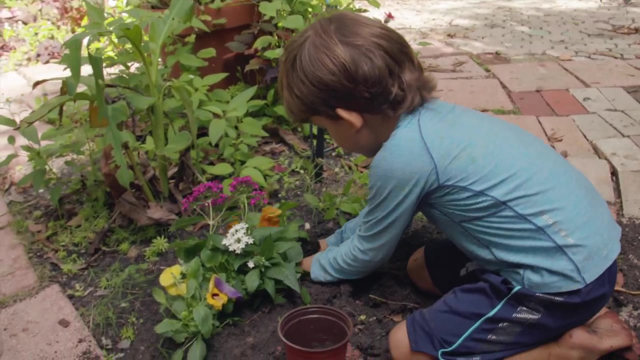 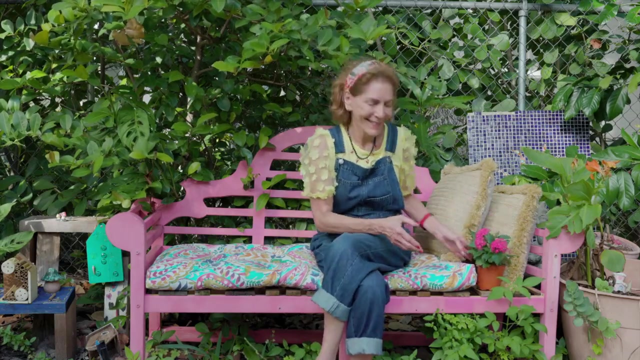 Let's plant some flowers today. Let's plant right there. You're going to circle right, We're going to go together. Circle, Circle, Circle, Circle, Circle. They need water. putting it in nice, Hi Shiny. 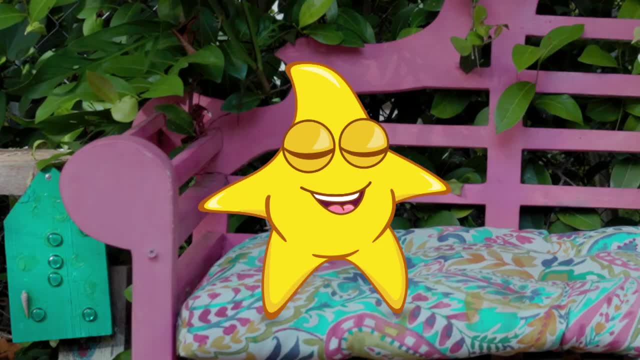 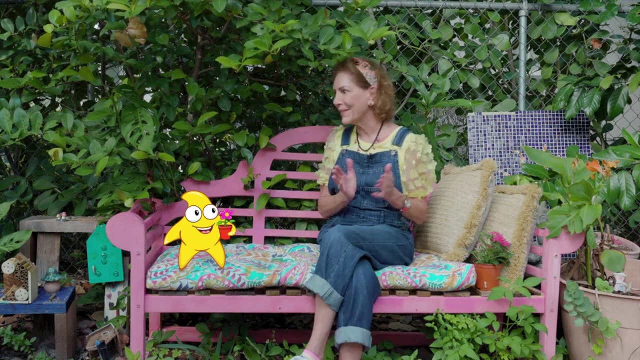 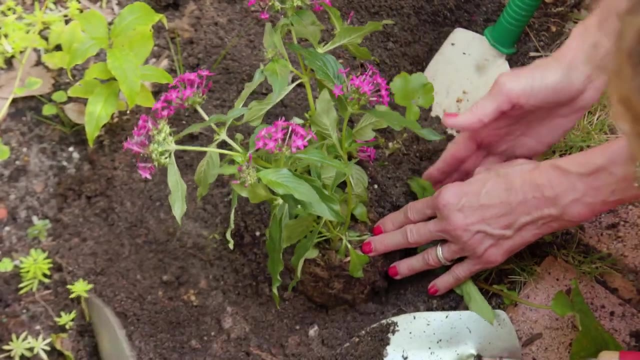 Would you like to help us decorate the fairy garden? That is a beautiful flower. I think it'll be lovely in here. I'm so glad you were able to bring us flowers. We need as many flowers as possible to fill this beautiful fairy garden with color. 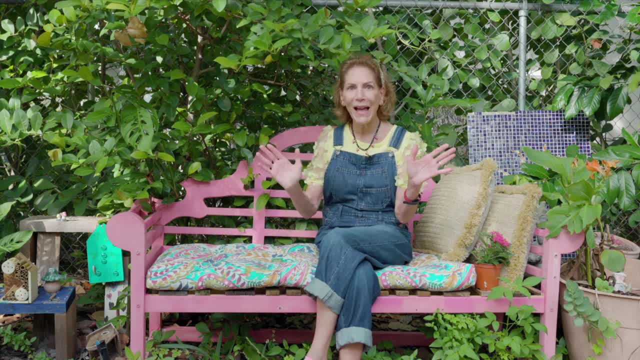 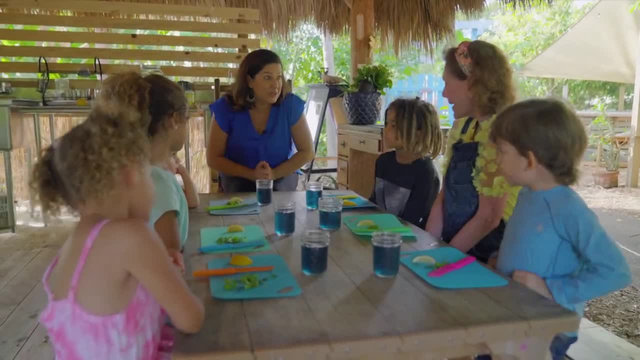 Ms Christina is gonna show us other great ways to use flowers. Let's go. So, Ms Penny, I brewed some butterfly pea vine tea for you to enjoy with the children. Oh, like the flower that we saw in the butterfly garden. 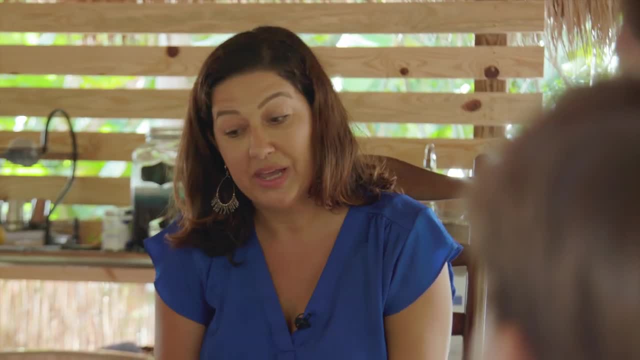 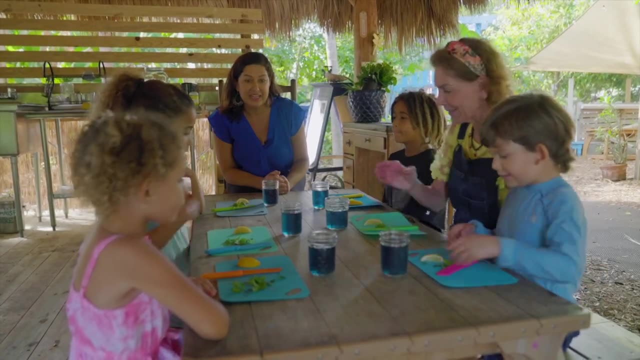 Just like that flower. So what you do is you dry those flowers and you can make a really nutritious tea out of them. You already dry those flowers And that's why they're there. look at it. Yeah, do you want to have a sip of your tea? 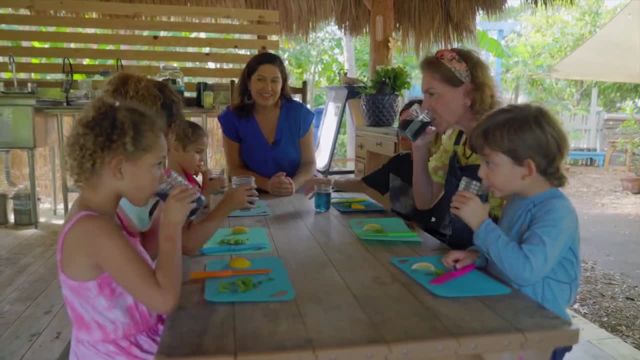 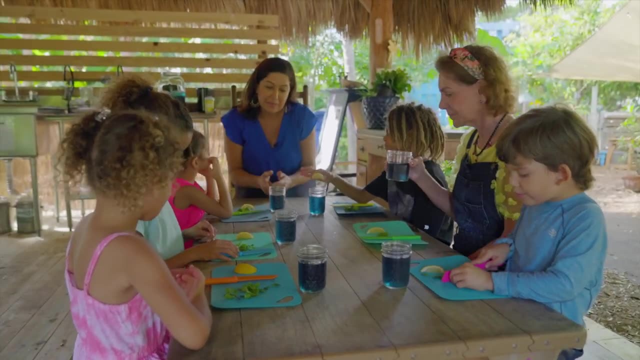 Yeah, Give it a little taste. Tell me what you think It's really good for your body. You can add a little honey to it, or maybe some mint and lemon. We have a little mint from the garden. You can give it a little swish and give it a taste. 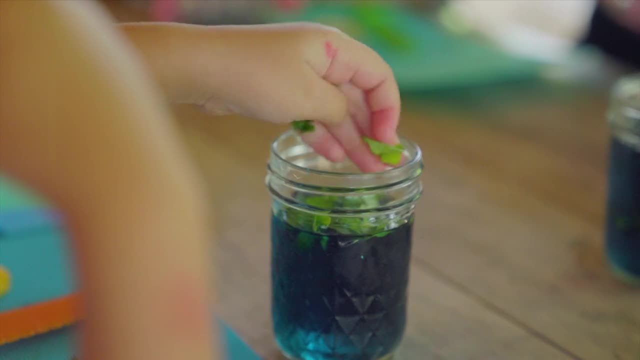 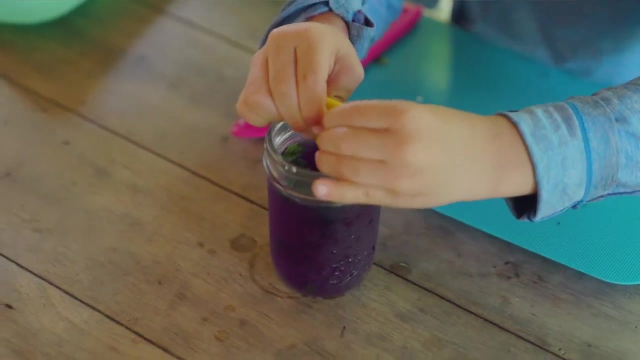 Tell me what you think. It smells delicious. It does smell delicious, It smells minty, It does Wonderful. So add some lemon. but observe what happens when you add the lemon: It turns purple. Oh wow, It changes the color. 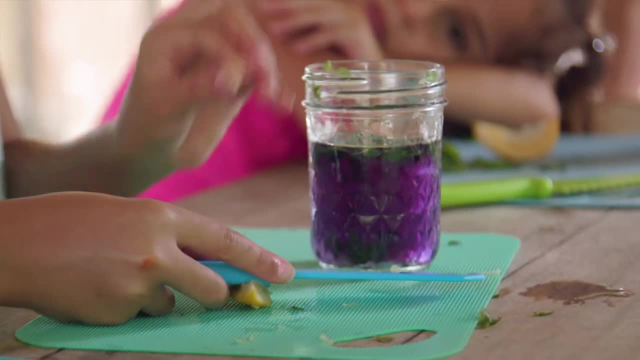 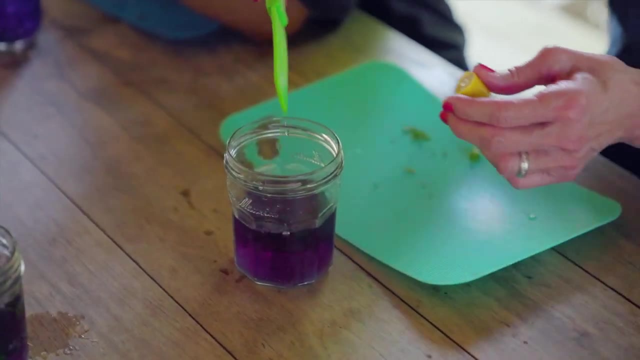 It does. Hey, how'd you do that? It's magic. Why is that changing? Add a little more lemon. see what happens. Ms Penny's turned purple too. It did. Mine's turned purple. It went from blue to purple and even pink. 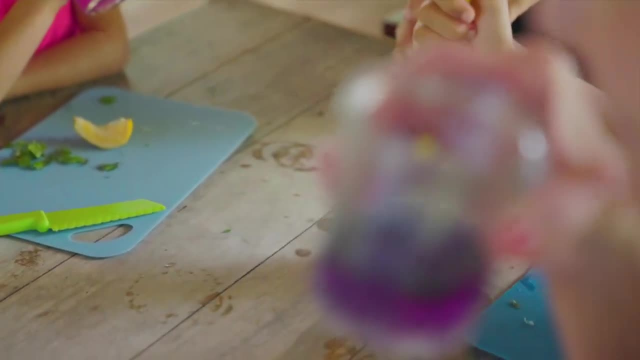 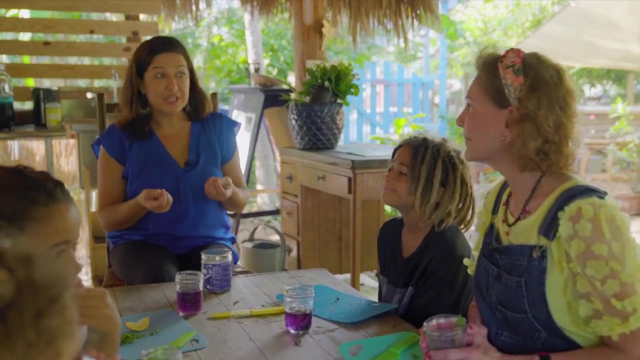 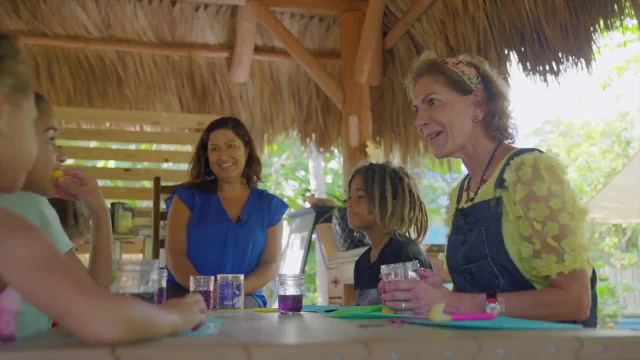 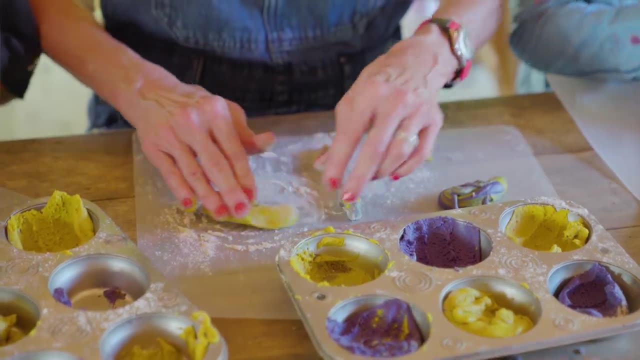 Oh, can we see that? Yeah, Do you want to play with Play-Doh? Yes, Yes, thank you, Let's do it. It's just flour, salt, and then I added a little water And for the coloring.